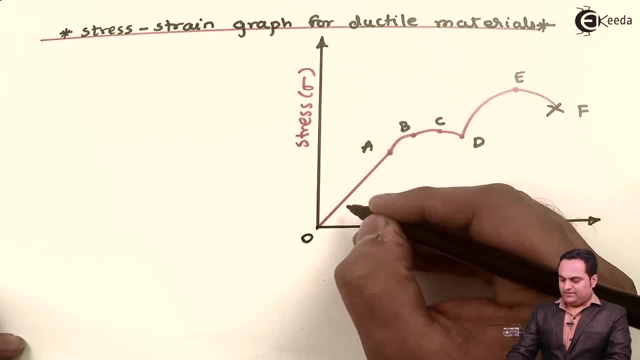 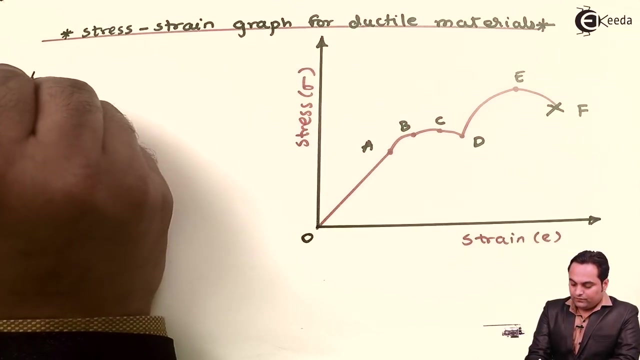 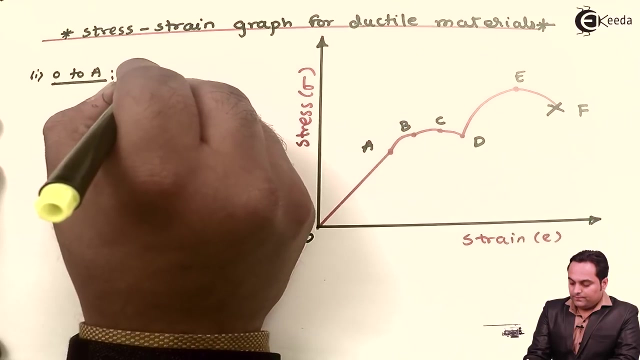 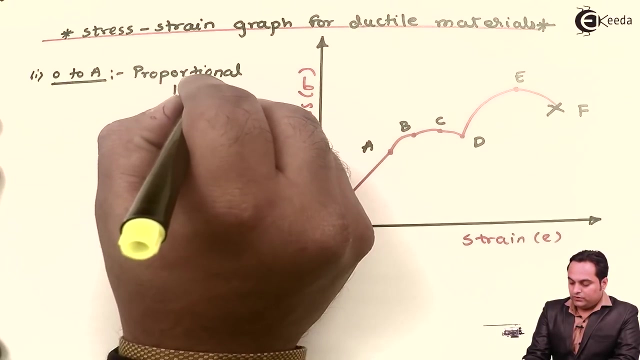 see, here we have an inclined line and this is we can say that since it is an inclined line, it is not a curve. So here we are getting a linear relationship between stress and strain, and I can say that here O to A, it is called as proportional limit. Now, when we say that, from O to A, it is: 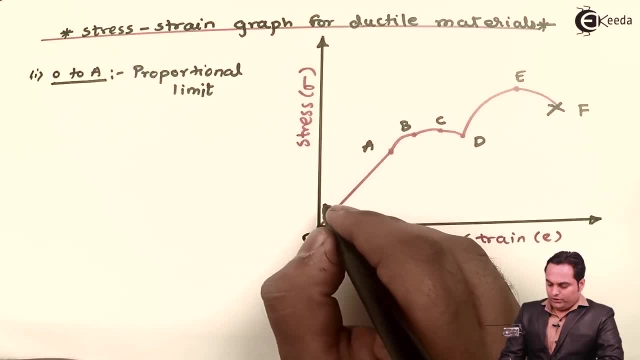 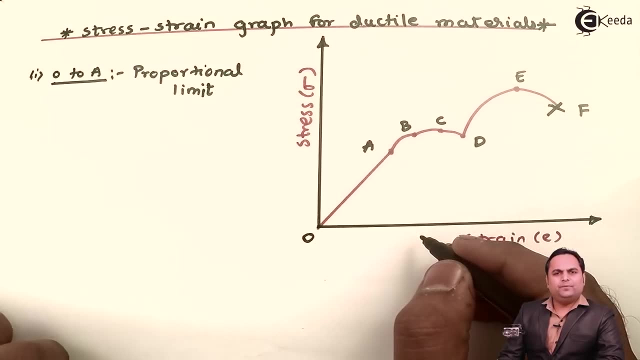 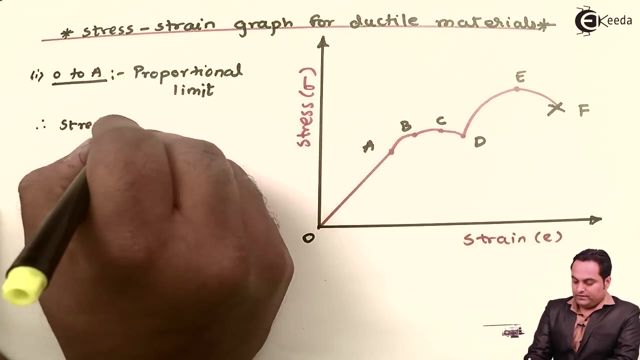 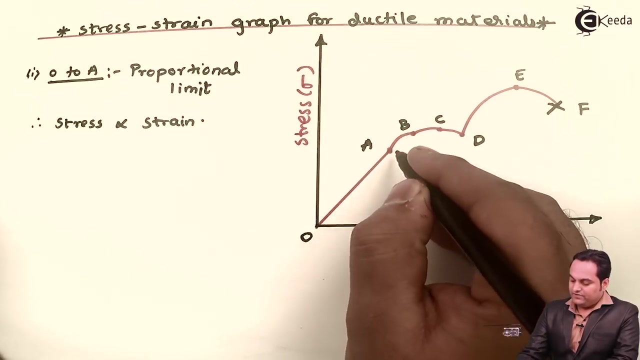 proportional limit. it means if we go on increasing stress, strain will also increase Means. the relation is directly proportional. So in proportional limit I can say that therefore, stress is directly proportional to strain. So now, as we can see in this stress- I have denoted it by Sigma Strain- it is: 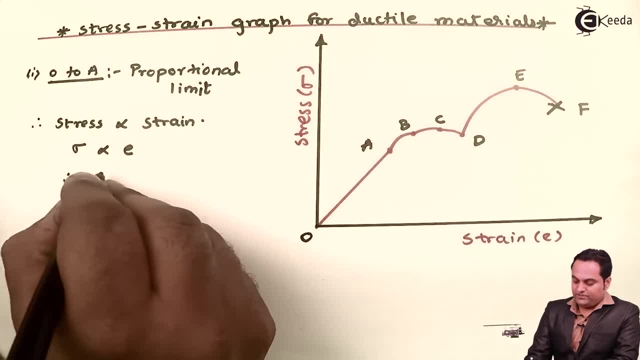 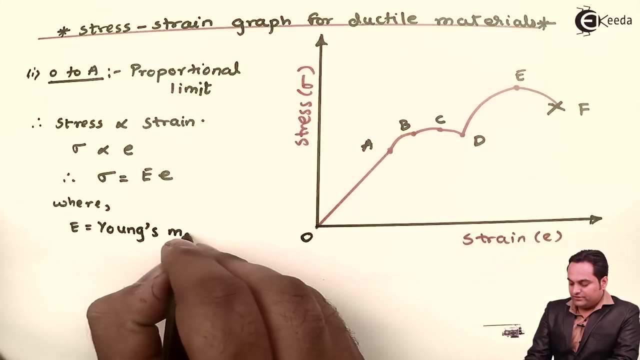 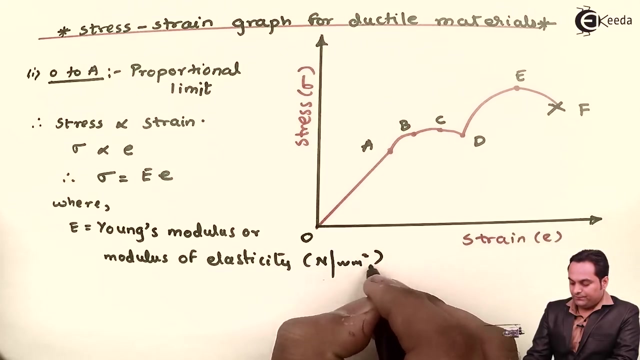 denoted by letter E. If I remove this proportionality sign, I have a constant here. It is called as E. I will say that where E is called as Young's modulus or modulus of elasticity, It's unit is Newton per mm2.. So, as we have seen in this graph from O to 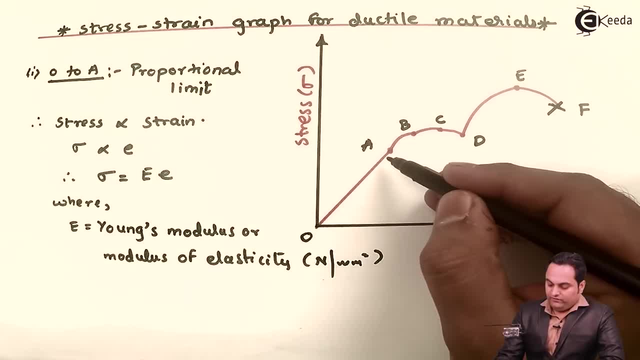 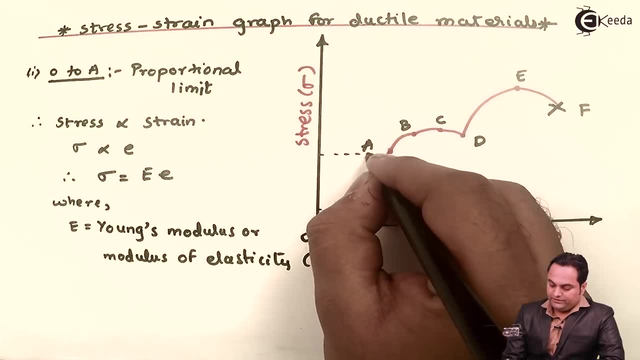 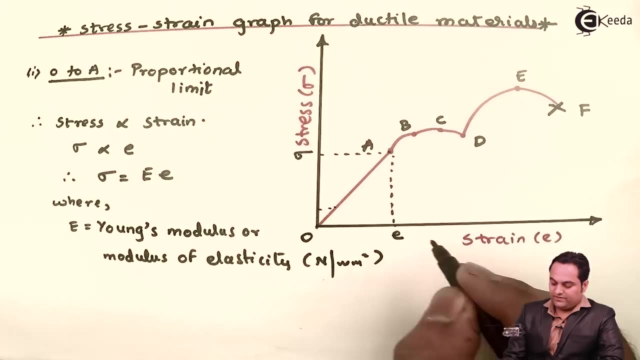 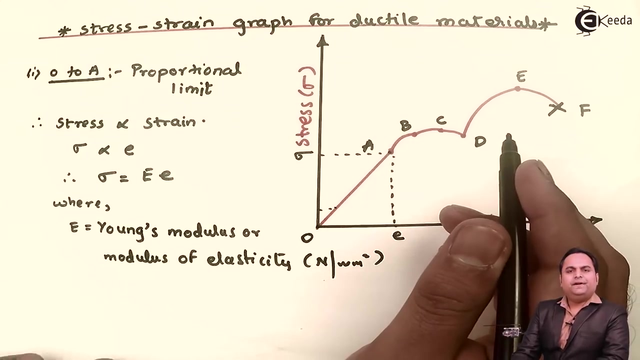 it is proportional limit. now when we reach point A, that is, if we are increasing the stress and we reach up to point A, then we are getting a strain value as well. here there will be stress and here we are getting strain. now, the moment we remove the load from point A, it means stress becomes zero. so if I 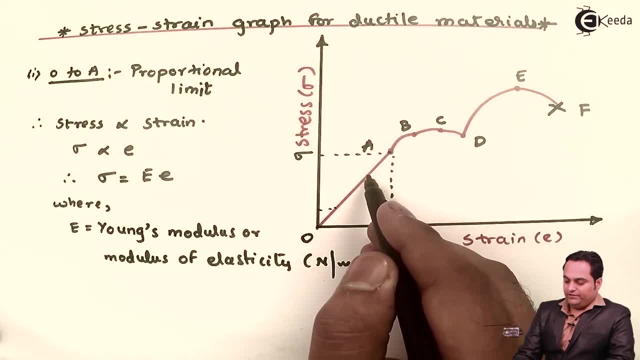 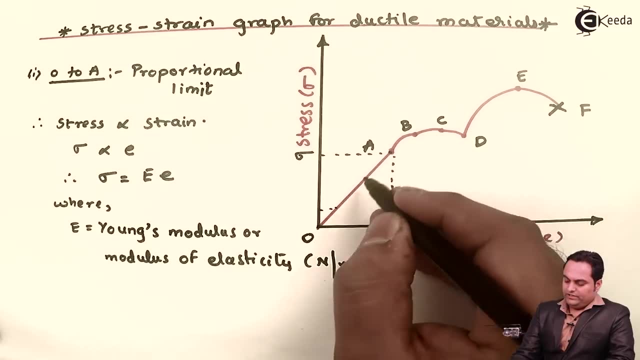 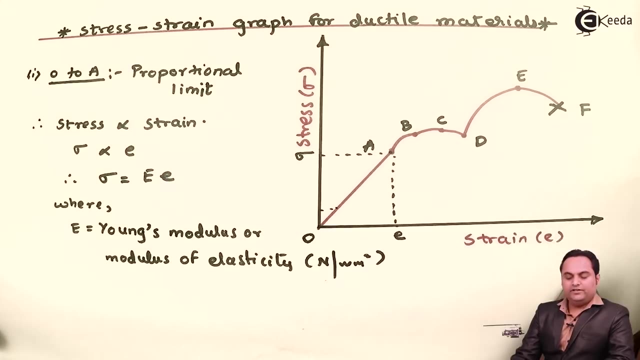 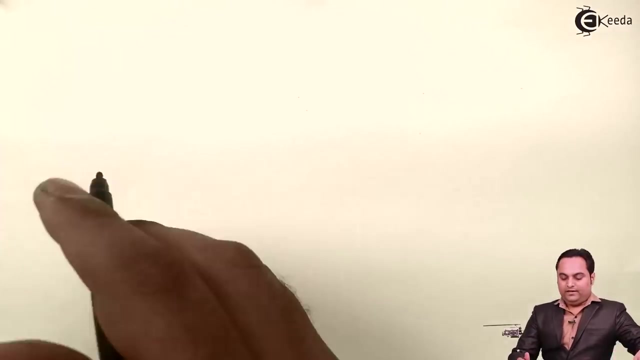 remove the load, this object will return back to its original shape. it means it behaves in an elastic manner. so within this 0 to a region the material behaves in an elastic manner. that is, when the load is removed, it will regain its original shape. next we see point A to B, that is- I'll write it down here- on the 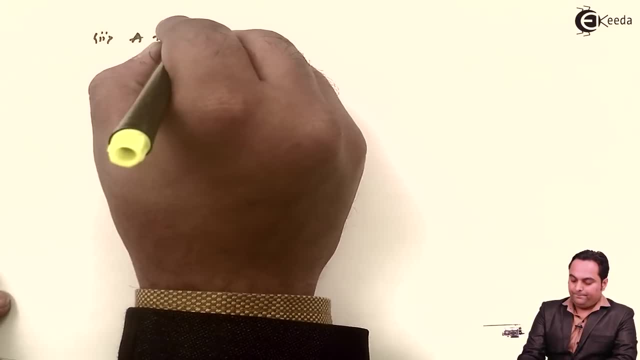 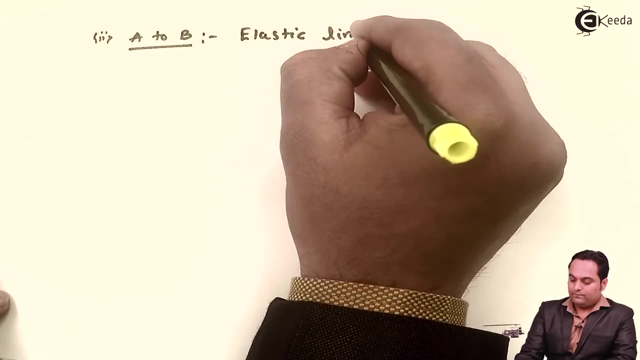 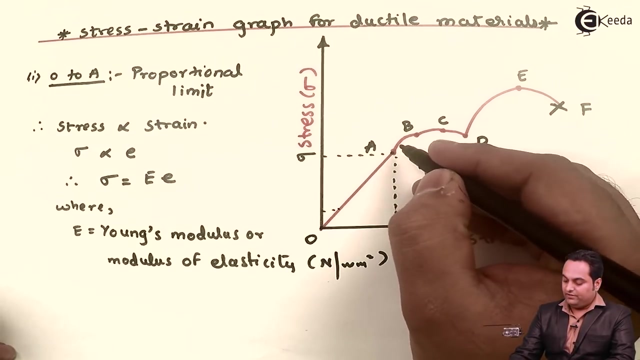 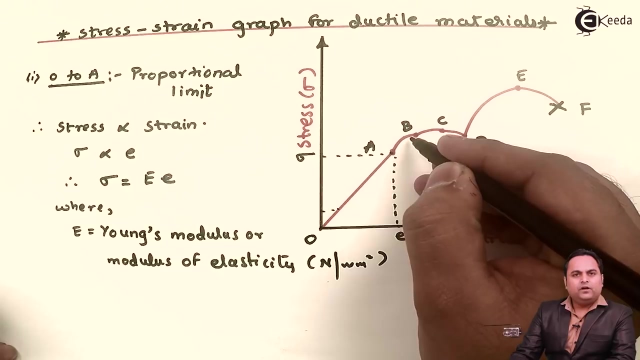 next page: from A to B. it is called as elastic limit. now, when I talk about elastic limit from A to B- again, as we can see here, that have when we have reached point B, from A to B, it is a curve. now, from 0 to A, the relation between stress and strain was linear. 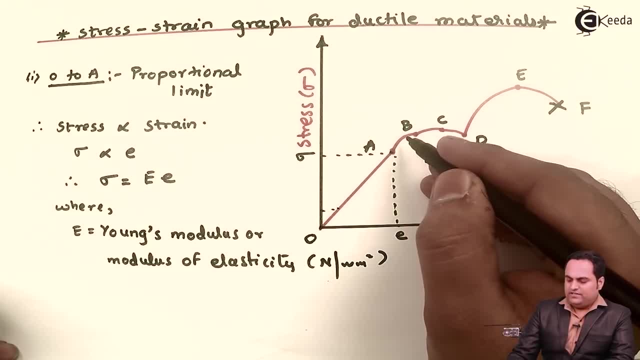 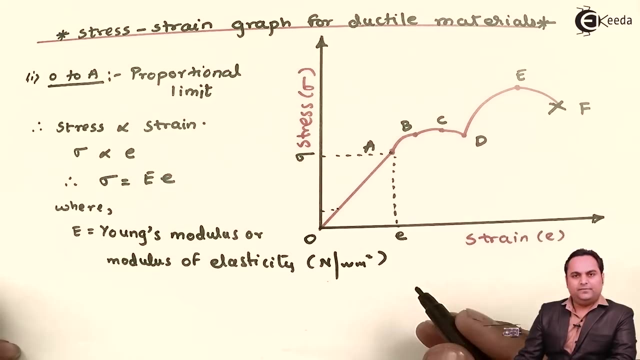 from A to B the relation is: it is a curve, so the relation is not linear like it was from 0 to A. but even at point B, if we are removing the load, the material will regain its original shape. so from A to B it is elastic limit. now when we go from point B to C, the change in stress is not. 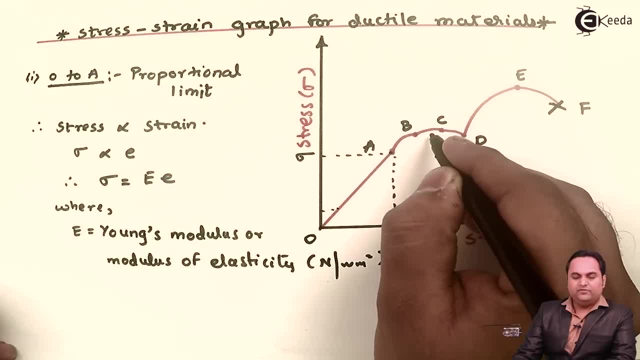 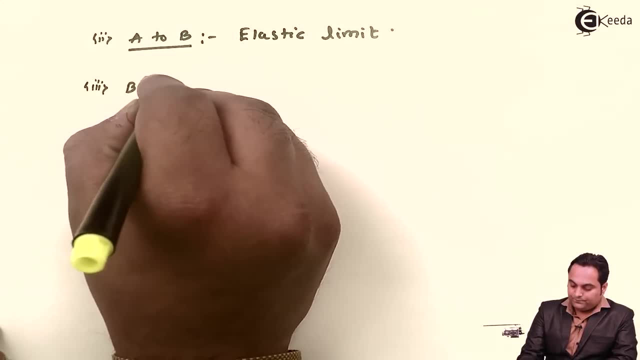 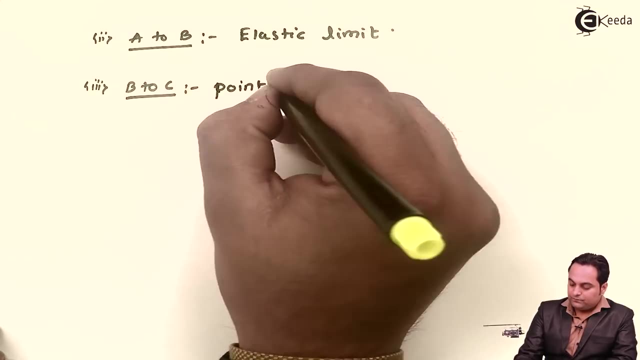 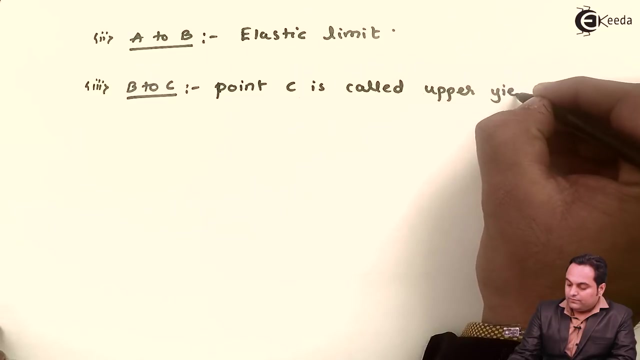 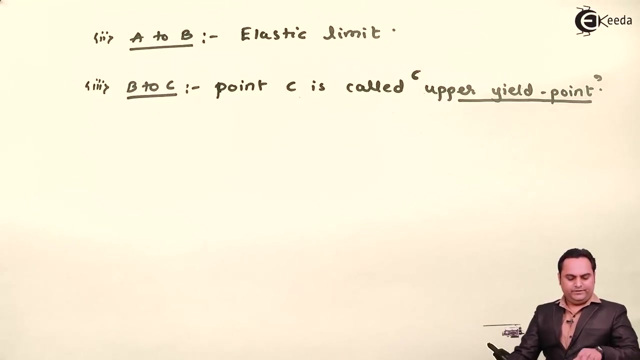 very much. as we can see, there is very little difference between B to C, so I can say that B to C it is called as here. I'll say that point C is called upper yield point. is called as upper yield point, it means at point C the yielding has started yielding. 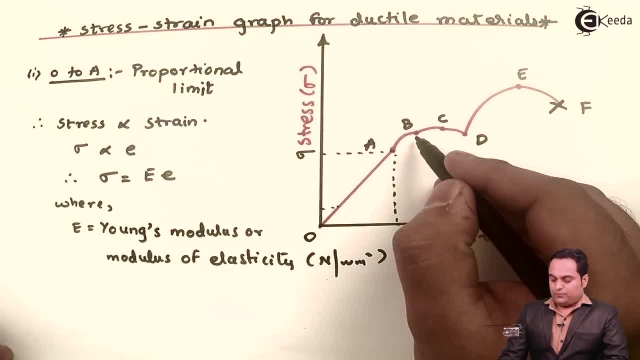 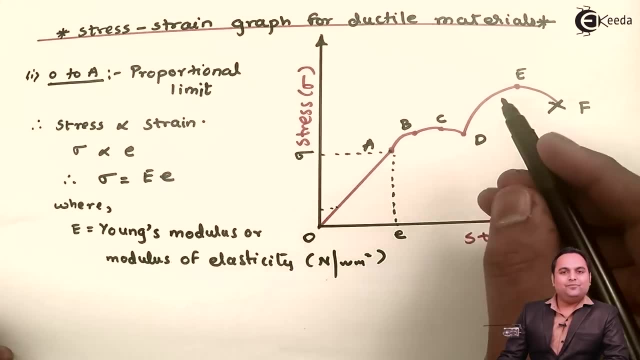 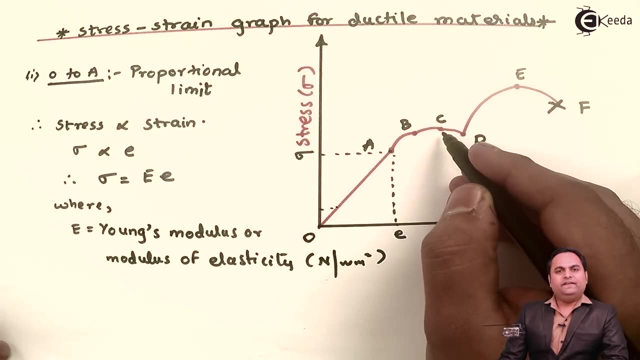 means change in shape. so once the material crosses point B it reaches in the region between B to C where it will be permanently deformed. that is, if we remove the load from point C then the material will won't regain its original shape. it means at point C it has deformed permanently. so this B to C 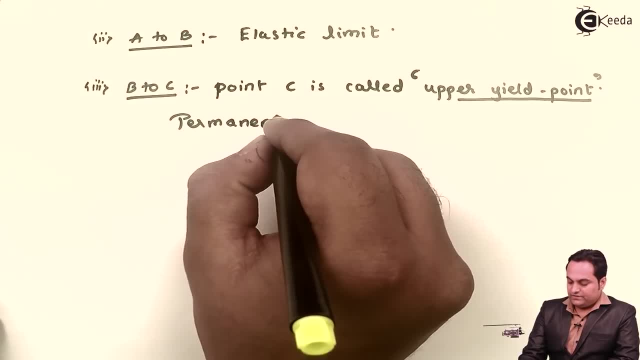 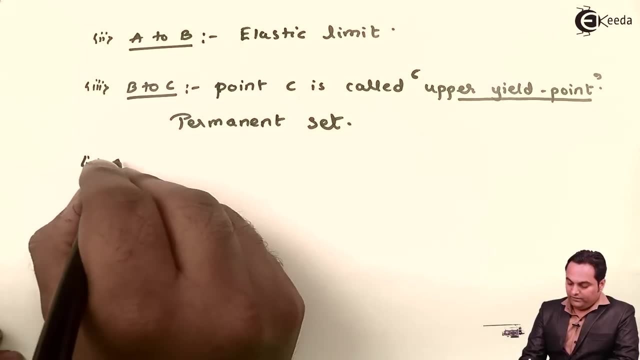 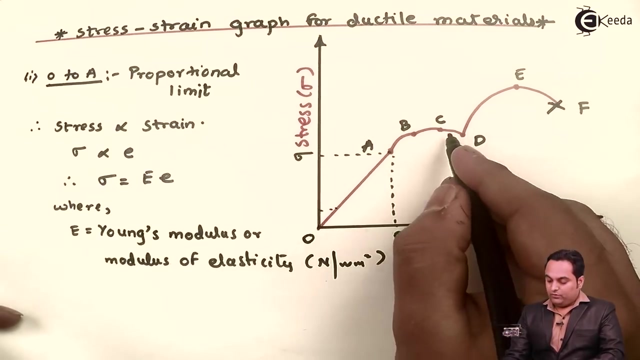 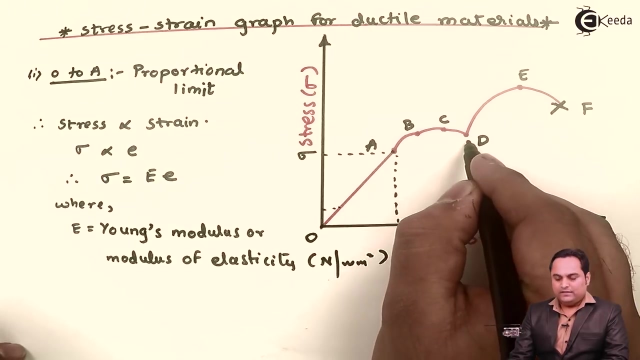 region. it is also called us permanent set. now, when we are from region C to B, is field is changed: region C to D. as we can see in this diagram. now, compared to point C, point D is below. it means the stress at point D. it is less compared to point C but the material is deforming more, as we can see. 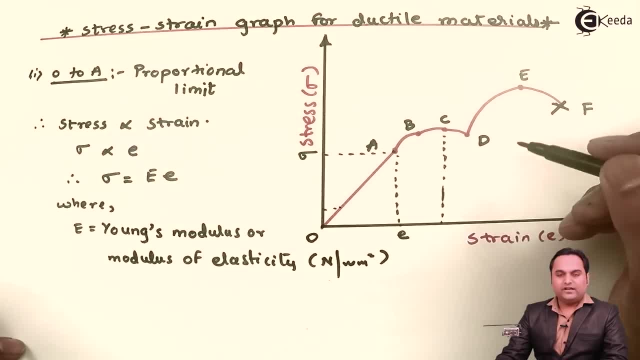 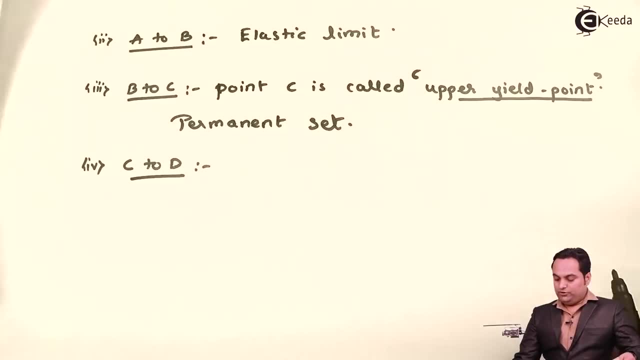 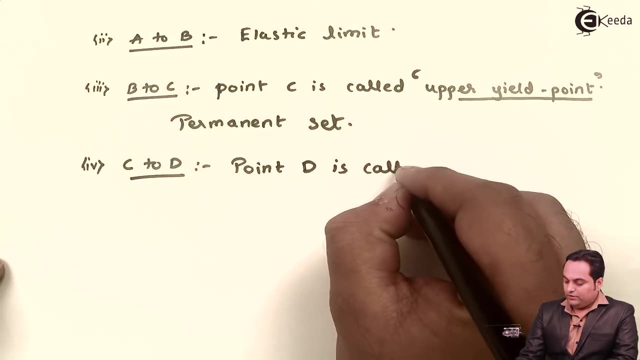 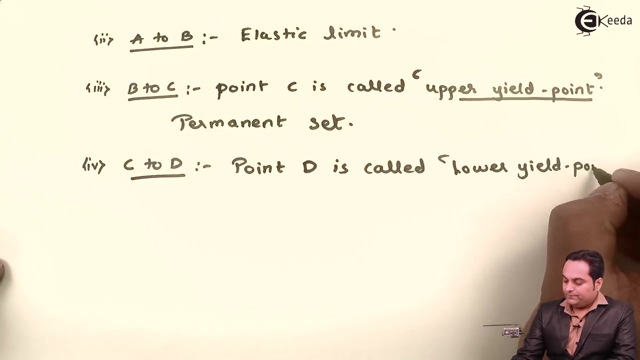 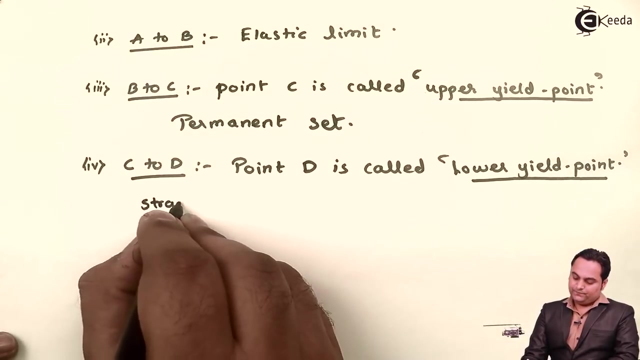 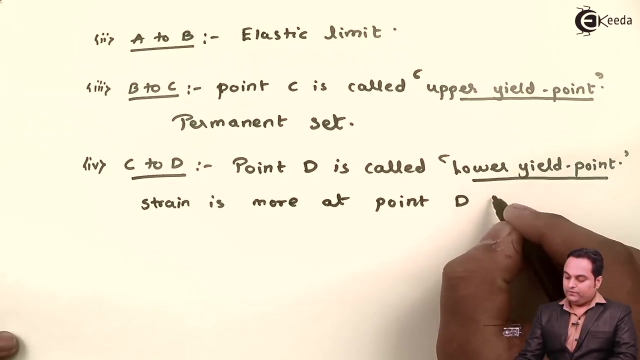 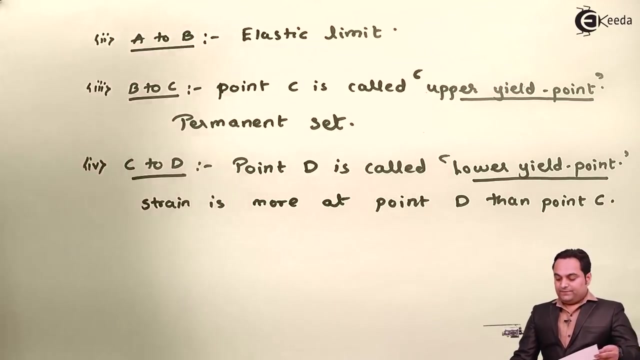 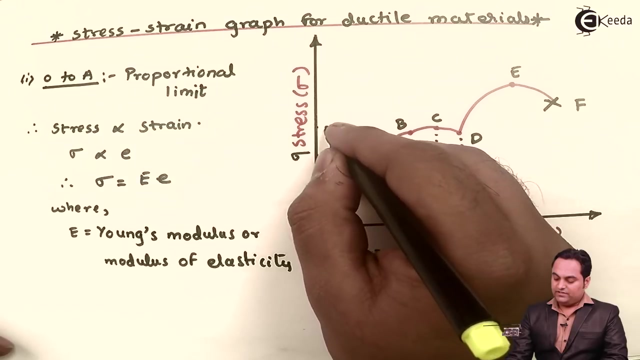 at point C the strain is less, strain means the physical deformation, and at point D the strain is more, but stress value is less. so here I can say that C to D. point D is called lower yield point, and strain is more at point D, then point C. next, as we can see in this diagram, D to E. here again stress is increasing. in a 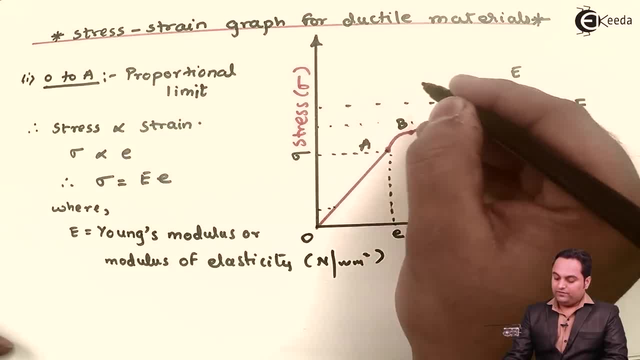 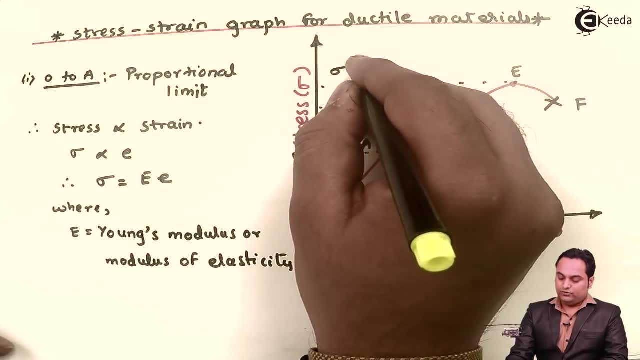 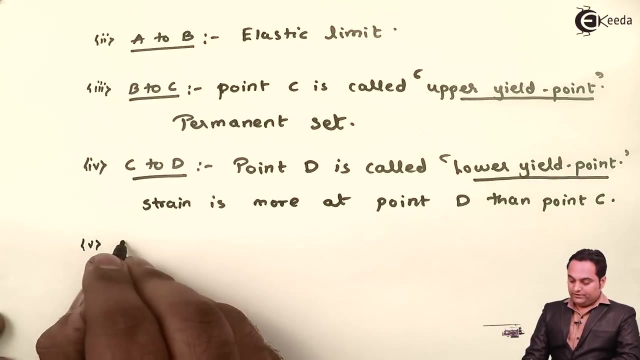 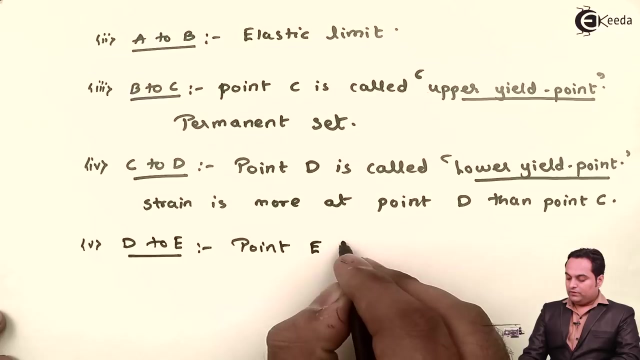 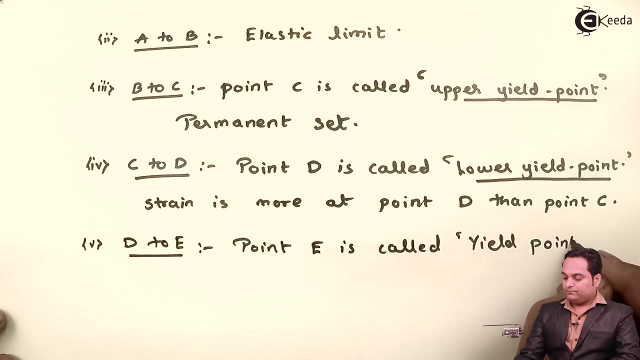 tremendously high manner, as we can see here. we can look at the diagram: the stress at point E. it is the highest point in this graph. so here we are getting maximum stress. so I'll say that point from the region D to E. your point E is called yield point and 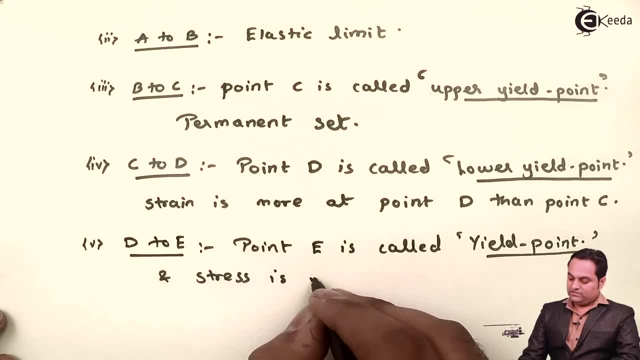 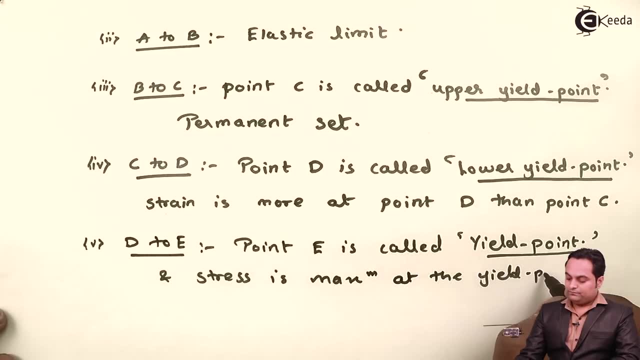 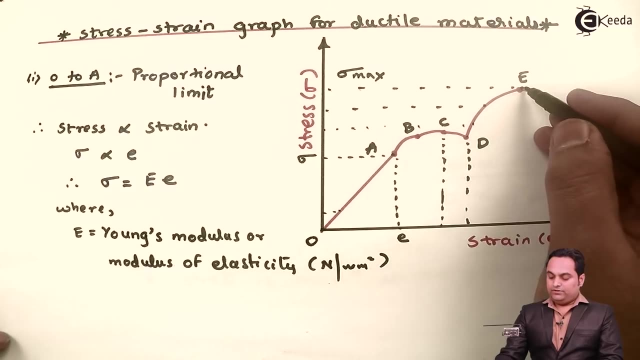 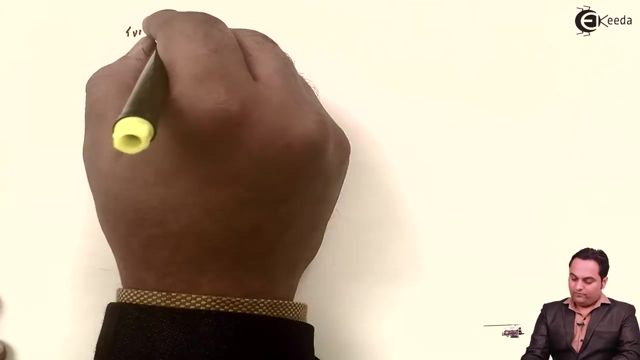 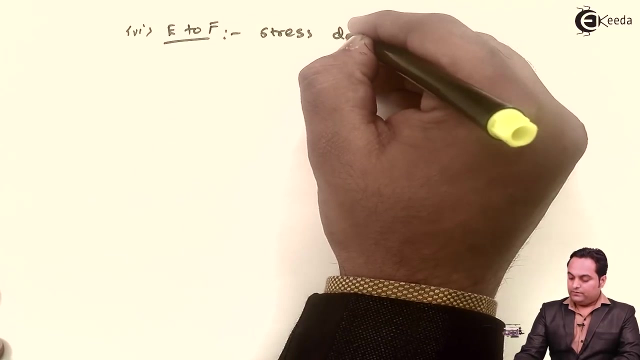 stress is maximum at the yield point. now, up to point, either stress is maximum, then if we go from e to F, the stress will go on reducing. as we can see, the graph is falling, so your stress decreases and from E to F we can say that stress decrease is. 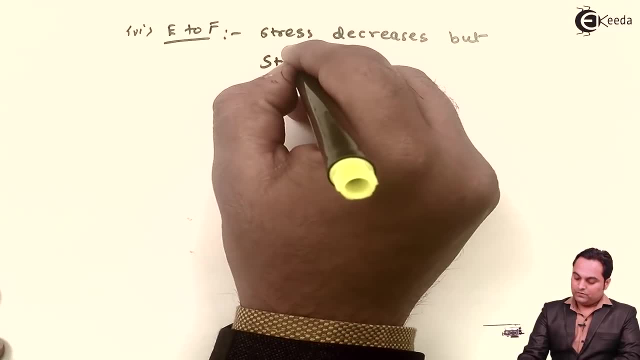 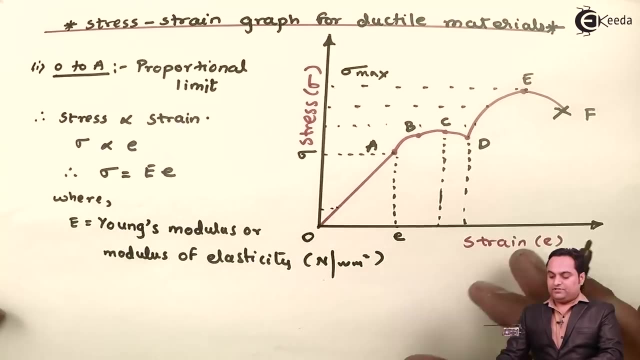 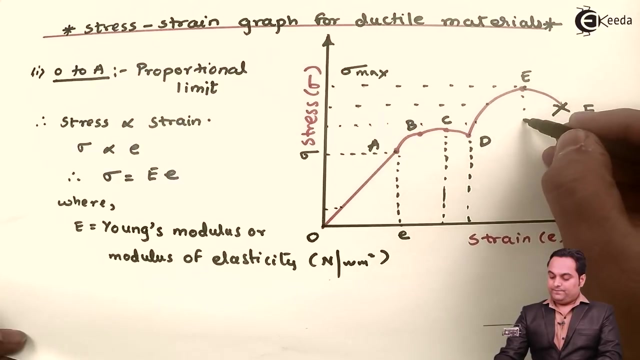 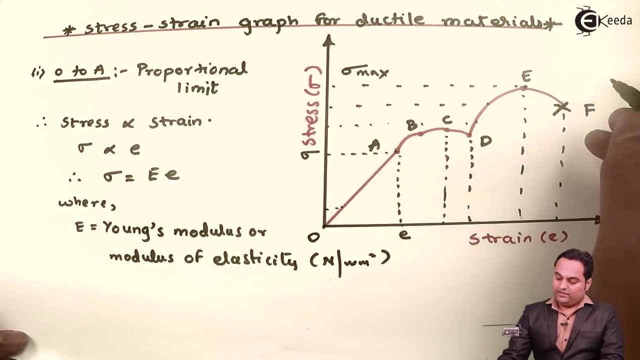 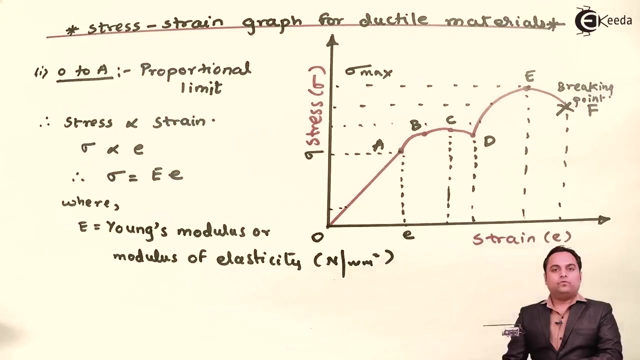 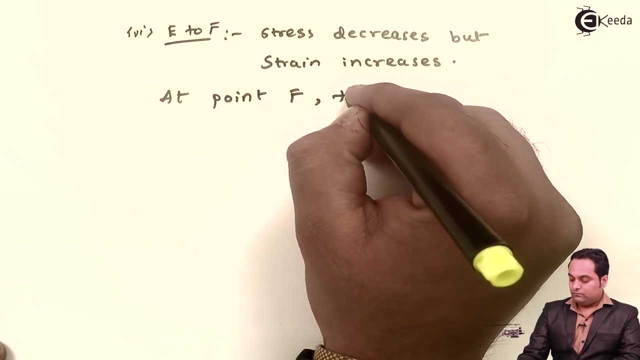 but strain increases. as it is very much clear from the diagram, from E to F the stress is falling whereas the strain is increasing. here we can look at this. and finally, at point F- here I have marked star- the material will be breaking and this is called as breaking point. so I'll say that at point F the material breaks.